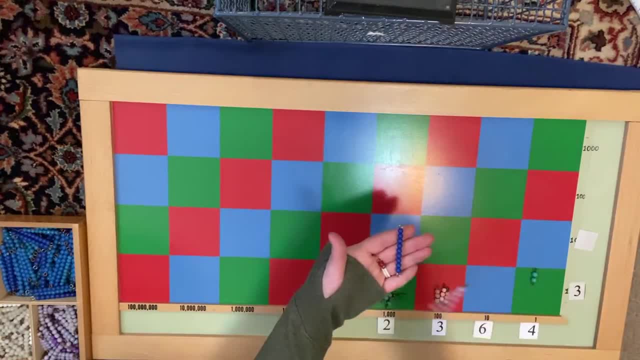 nine. I'm gonna take these out. whoa, that one things. that's crazy. the nine goes in the square we were counting and the one goes next door. okay, so now we're going to do this. one, three, six, nine plus one is ten. hmm, I want you. 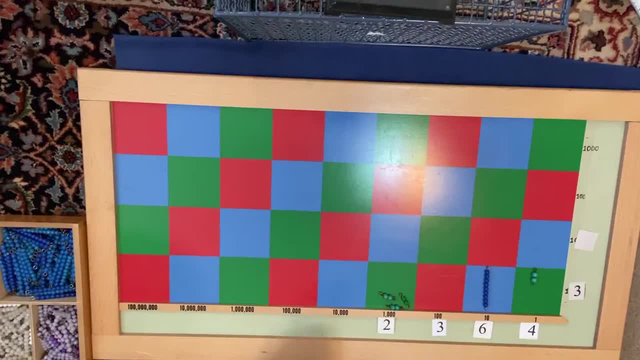 to picture the number ten: It's a 1 and a 0, like this right: The 0 goes in the square you counted and the 1 goes next door. And to represent a 0 with beads, we just don't put anything. 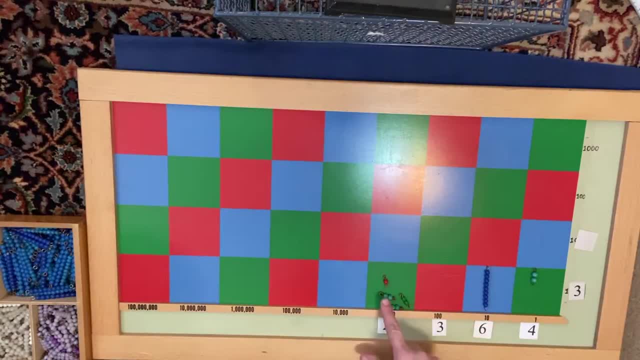 Okay, so now we have this: 2,, 4,, 6, plus 1 is 7.. That's just a one-digit answer, so we only need one square for that. Okay, so we have our first partial answer. 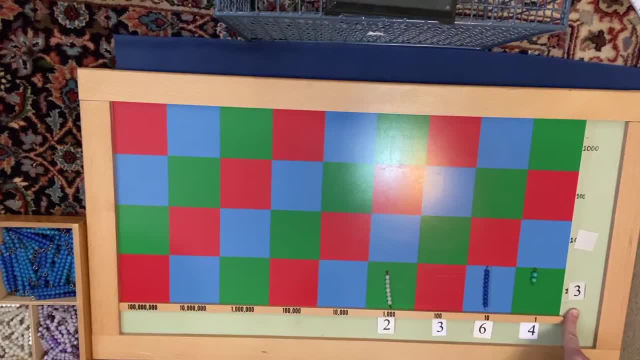 And remember, an answer to a multiplication problem is called a product. So we have our first partial product. Okay, we're going to flip this over. I'm going to flip the 4 over, And here we have to start on this row. 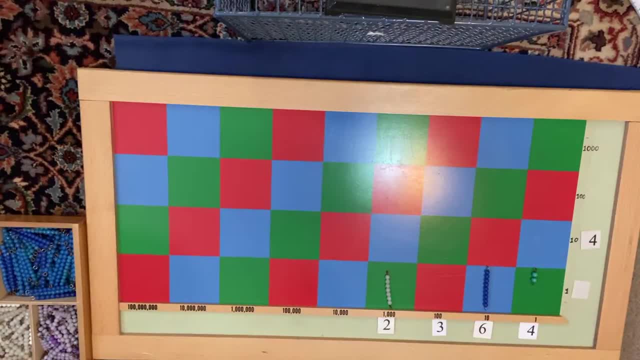 Okay, so 4 times 4.. Crazy, crazy beads. 4 times 6 is going to be there. Whoa Oops, I only have 3.. One more 4 times 3 goes right here And 4 times 2.. 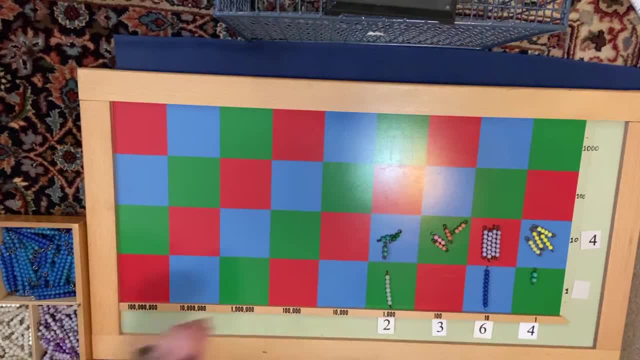 Okay, so we're going to start over here and we're going to do some counting: 4, 8, 12, 16.. Picture 16 in your head: A 1 and a 6. This number goes in the square. we counted. 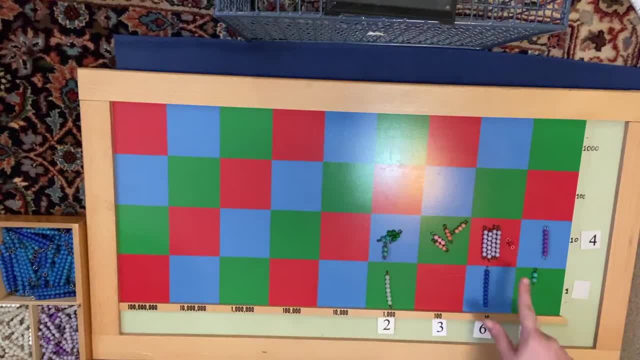 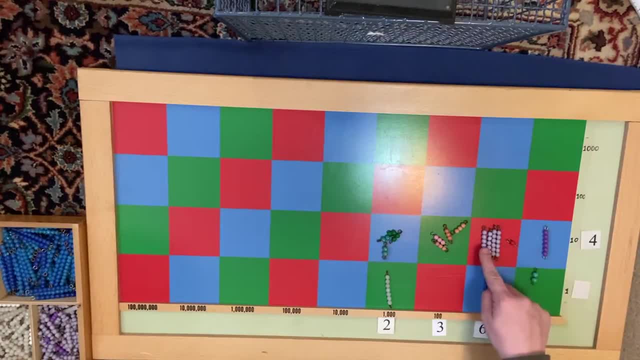 Okay, now we're going to add all this together: 6, 12,, 18,, 24.. Plus 1 is 25.. So we're going to picture 25 in our heads: A 2 and a 5.. 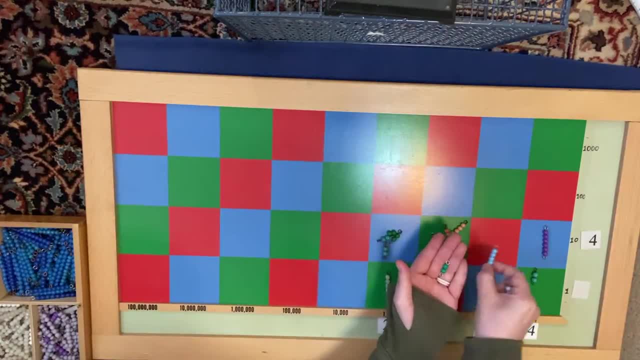 Take these out. The 5 goes in the square we counted And the 2 goes next door. Oh, it's rolling away, Crazy 2.. Right up there, Okay. so let's count 3,, 6,, 9,, 12,, 13,, 14.. 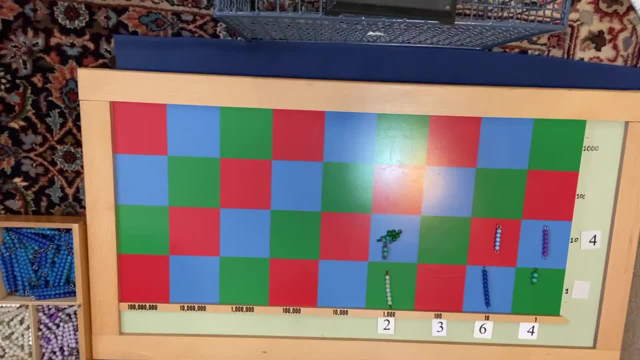 So picture a 14 in your head. It's a 1 and a 4.. Like this, The 4 goes in the square we counted And the 1 goes next door. Wow, that square really likes to have beads roll, doesn't it? 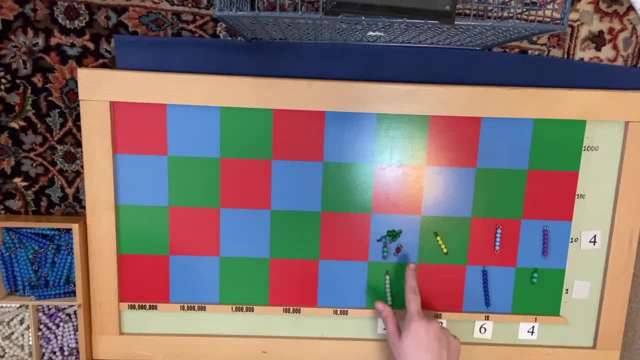 Okay, and then we're going to add these 2,, 4,, 6,, 8,, 9.. Whoa, Okay, So we have our second partial product all multiplied and ready to go. Now do you remember before when we would always read answers? 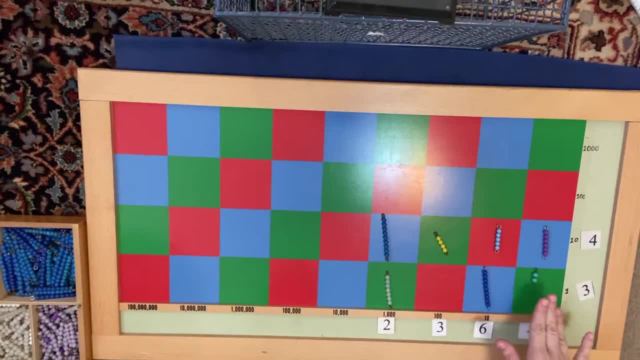 everything was down here On this bottom row. Well, that still needs to happen. So I want you to watch carefully what I'm going to do. I'm going to combine my like categories. That means this is a 10 and this is a 10.. 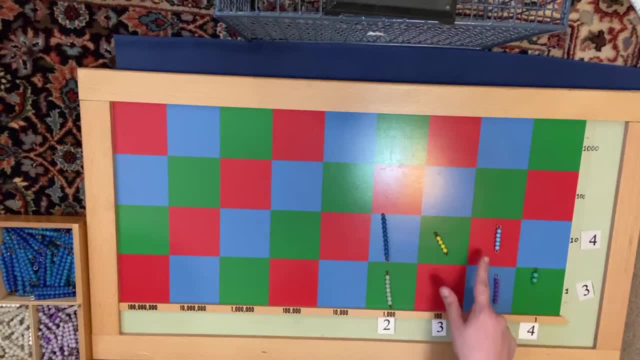 So I'm going to slide this down. This is 100 and this is 100.. I know there's nothing there, but it's still 100.. I'm going to slide this down. This is a thousand and this is a thousand. 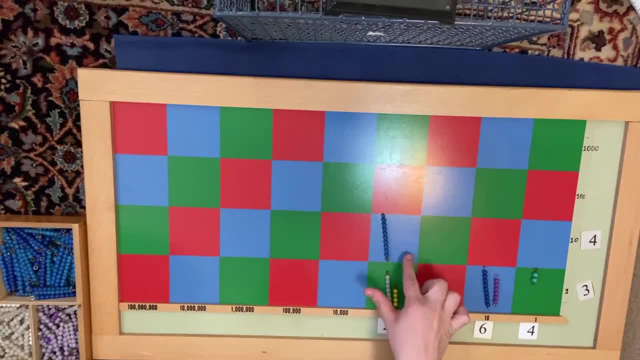 I'm going to slide it down. this is a 10,000, and this is a 10,000.. I'm going to slide it down. okay, And now we have one more thing to do: We need to go back and make sure there's only one bead bar in each square. So do. 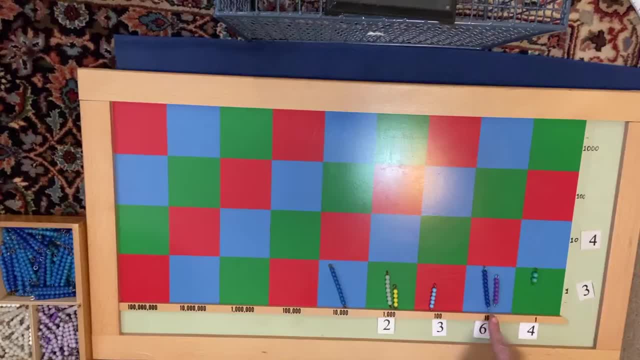 we have one bead bar here. Yeah, that's the number two. What about here? We have two bead bars, don't we? So we need to add them together. So this is nine, 10,, 11,, 12,, 13,, 14,, 15.. So picture 15 in your. 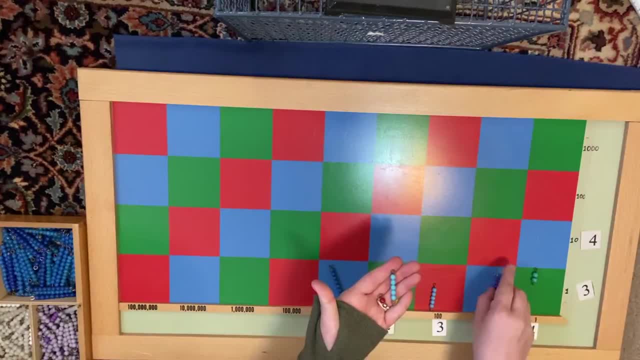 head: a one and a five. This number goes in the one we counted. This number goes next door. Okay, so we have one bead bar there. Look here. Oh, now we have two. Five plus one is six. Put that there. Now let's go here. Seven, eight, nine, 10, 11.. Picture 11 in that head of yours. 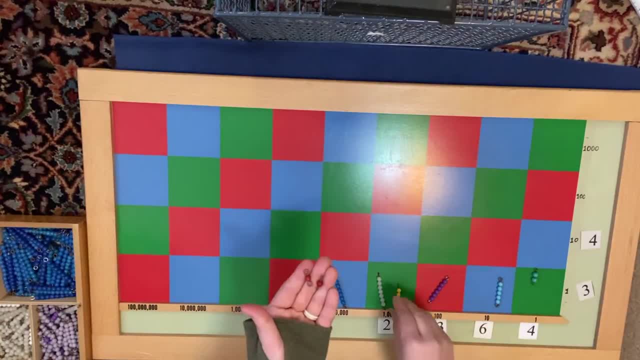 What two little digits do we use to make that number? A one and a one. This one goes here, This one goes next door. Okay, now we just have to add these two, Nine, 10.. Oh, there's another 10.. So picture 10 in your head. What does it look like? 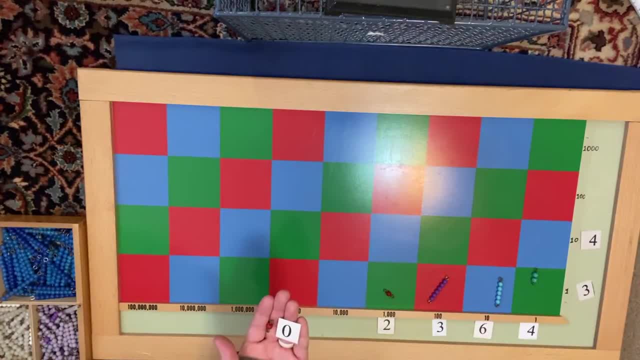 It's a one and a zero. This number goes in the square we were counting. This one goes next door. Remember the way we represent zero with beads? is we just put nothing? So we have our answer. So we're going to just look at this right here: 110 unit. 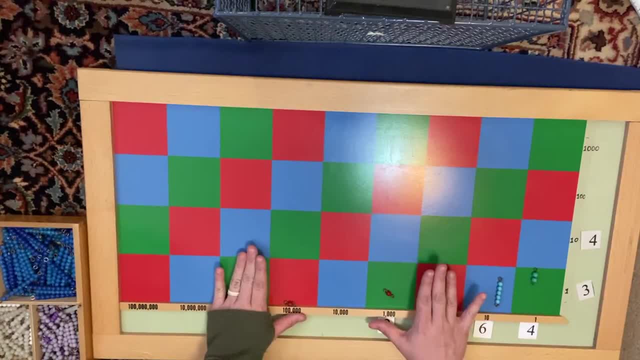 This says 101,000, because this is the thousand family: 652.. 2,364 times 43 equals 101,652.. Awesome, Let's do another one and get reset here. Okay, you guys. So we're going to multiply 8,327.. 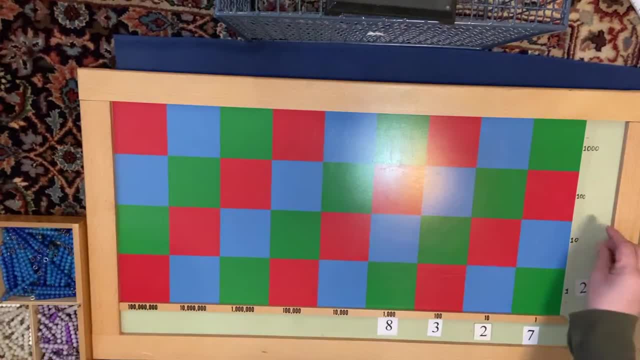 By 32.. Okay, so again, we always start with the units, So we're going to multiply everything down here by two, So two times seven. This time, instead of setting out the actual two sevens, I'm going to show you what it looks like to just set out the answer. 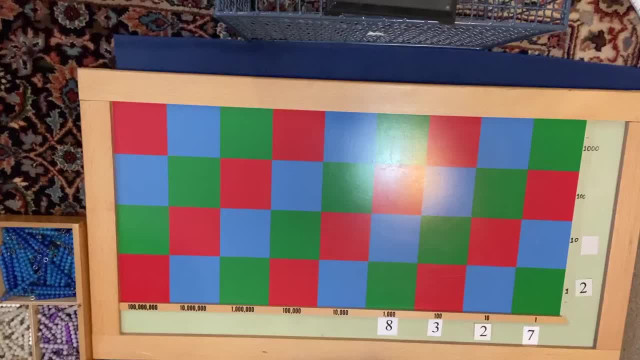 So two times seven is what It's 14.. So again, picture 14 in your head. It's a four and a one. This goes in the square we were counting and this goes next door. Okay, 14.. Two times two. What's two times two? 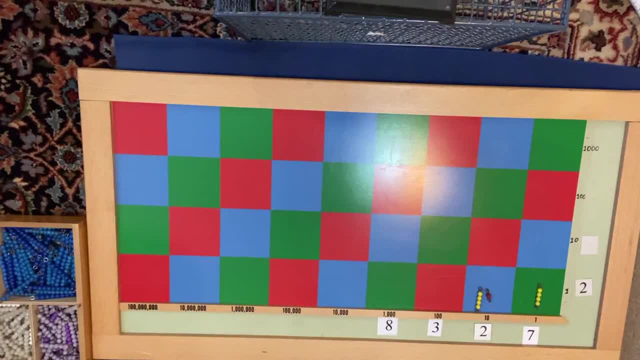 Four. Now, if you wanted to, you can add this up, but I'm going to wait to do that until the very end. Two times three is what Six. Two times eight is what Sixteen. So picture sixteen in your head. 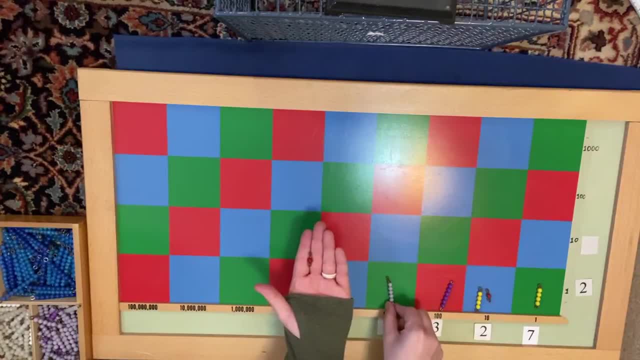 It's a one and a six. Six goes in the square- we were multiplying and one goes next door. Okay, so let's make sure there's one bead bar in each square. One, Oh, we need to do this. Four plus one is what. 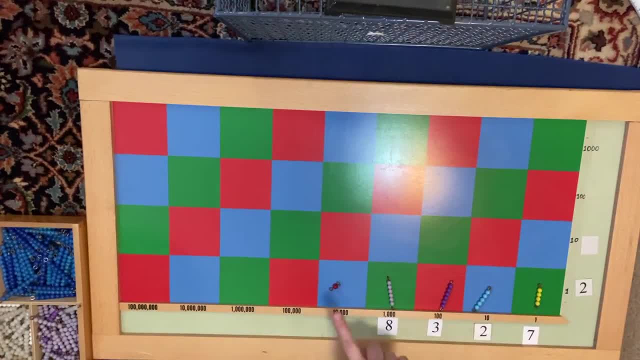 Five. And then we have one bead bar, one bead bar, one bead bar. Okay, that means we can go on to our tens place. So this says we have to multiply everything down here by three, So we have to do three times seven. 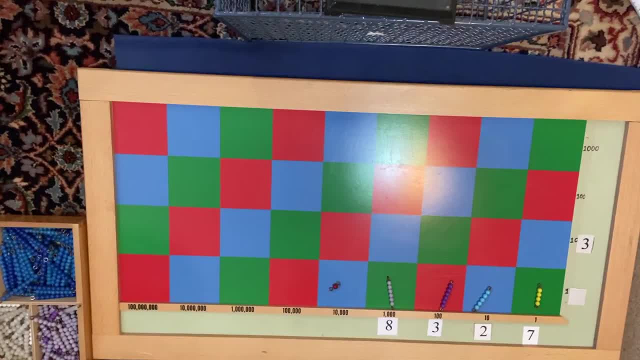 What is three times seven? Three times seven is twenty-one, So the one goes in the square. we were multiplying, the two goes next door, So now we need to do three times two right here. What is three times two Six Six? 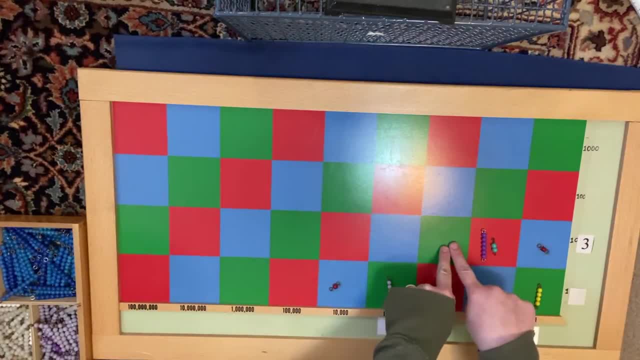 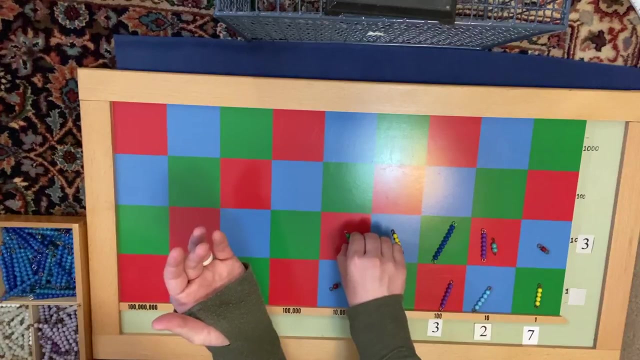 Now we need to do three times three, which is nine, And three times eight, What is three times eight, Twenty-four. So we put the four in the square we were multiplying and the two next door or ahead of it. Okay, so let's make sure we have one bead bar on each square. 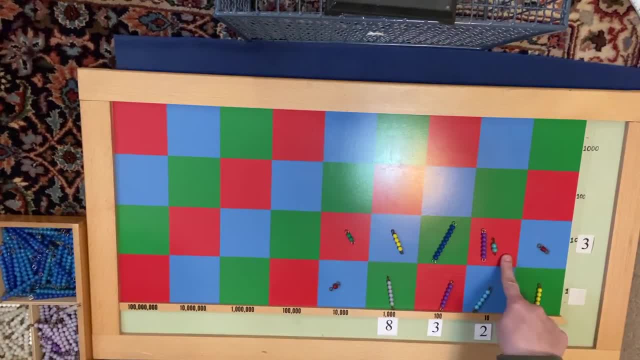 Square, or in each square up here, One bead bar, but here, And we've got to add them, Six plus two is eight, Cool. And then we have one bead bar, one bead bar, one bead bar, Cool. So now we need to slide the like categories together. 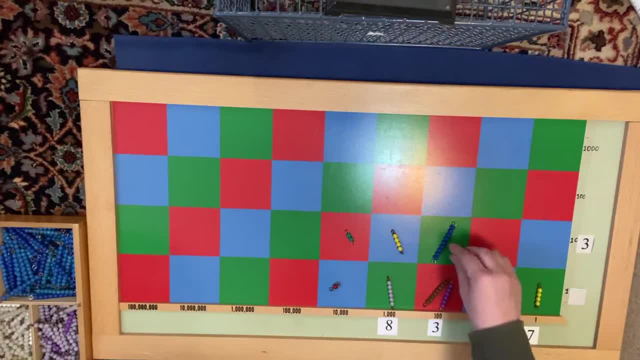 Ten with the tens, Hundreds with the hundreds, Thousands with the thousands, Ten thousands with the ten thousands, And look, We still don't even have a hundred thousand. We're getting some pretty big numbers, huh? So do we have one bead bar here? 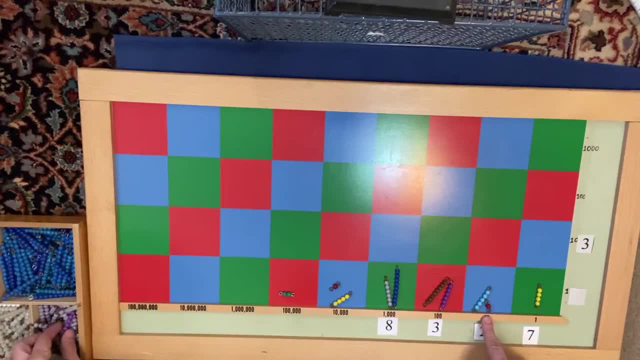 Yeah, What about here? Five plus one is six. Eight plus six is what? Fourteen Picture fourteen. The four goes in the square. we counted, One goes next door. Okay, now let's look at this. We have one plus nine plus six. 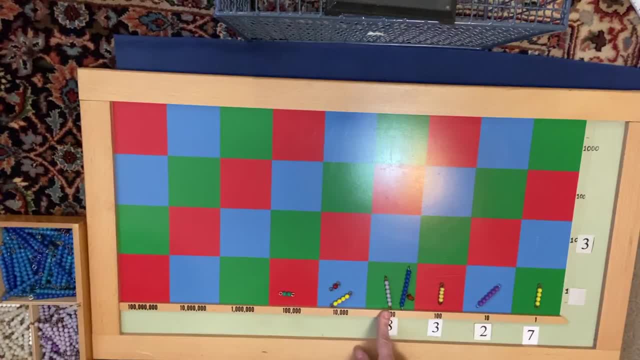 Well, one plus nine is ten. That's pretty easy. Ten plus six is sixteen. So picture sixteen in your head. One and a six. Six goes in the square. we were counting. One goes next door. So one plus one is two. 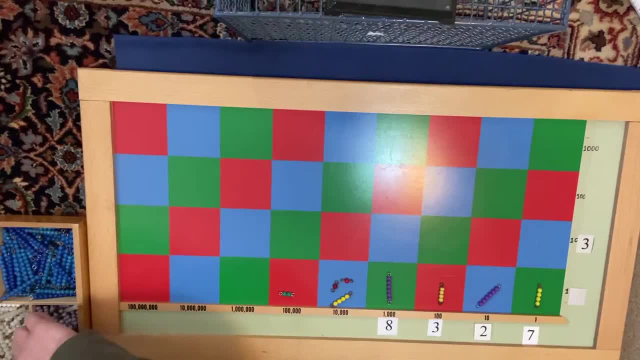 Two plus four is what Six, Another six, Six, Uh-oh, Crazy one. So we have our answer. Let's go ahead and read this. We start here: If it was just two, six, six, it'd be two hundred sixty-six. 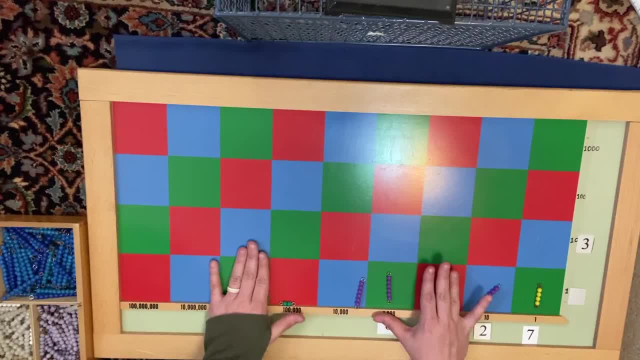 And what family is this? Thousands, So two hundred sixty-six thousand four hundred sixty-four, So eight thousand three hundred twenty-seven times thirty-two equals two hundred sixty-six thousand four hundred sixty-five, So that's three hundred sixty-four. 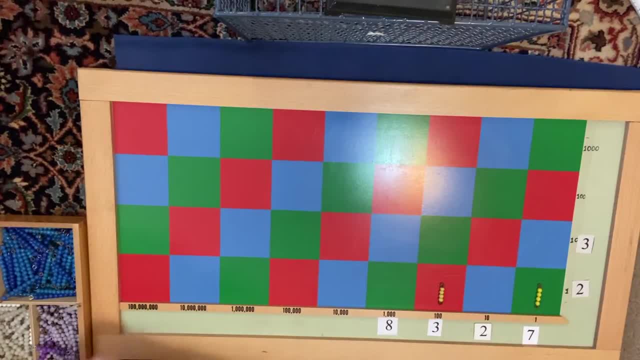 Good. Now say you wanted to do a problem that had three digits up here. Well, I'm going to show you how to do that. It's really not any different than what we just did. So we're going to multiply three thousand six hundred forty-two by four hundred thirty-two. 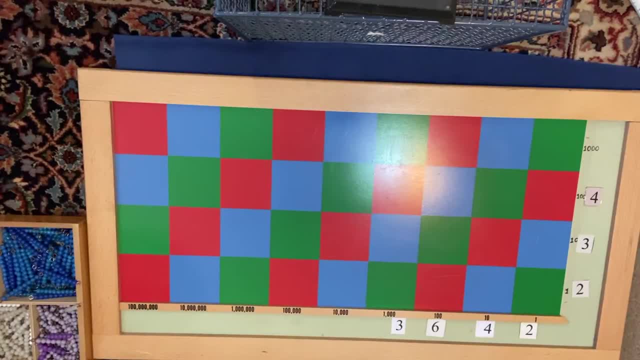 Sweet. So we're going to do the first two rows the same exact way we did it before. Okay, Everything down here is going to be multiplied by two. So two times two is four, Two times four is eight. Two times six is twelve. 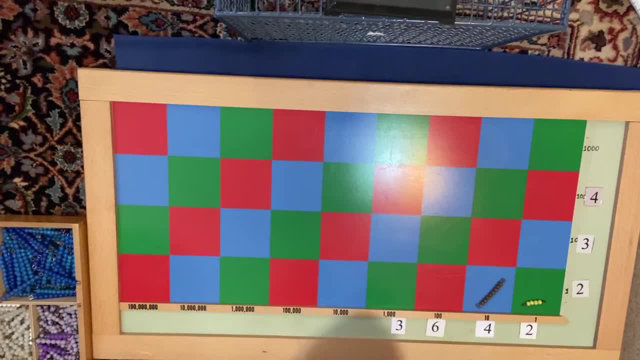 Picture twelve in your head: Two and a one. Two goes in the one. we were multiplying. One goes next door. Two times three is six. Let's make sure there's one bead bar in each square. One bead bar, Yes, One bead bar. 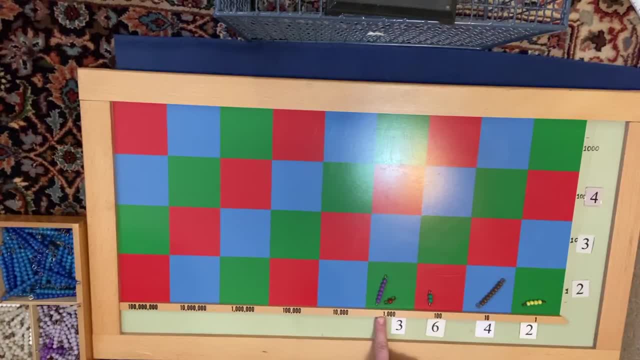 Yes, One bead bar. Yes, One bead bar. No, Six plus one equals seven. Now we have to go up here and multiply everything down here by three. So this would be three times two. What's three times two? 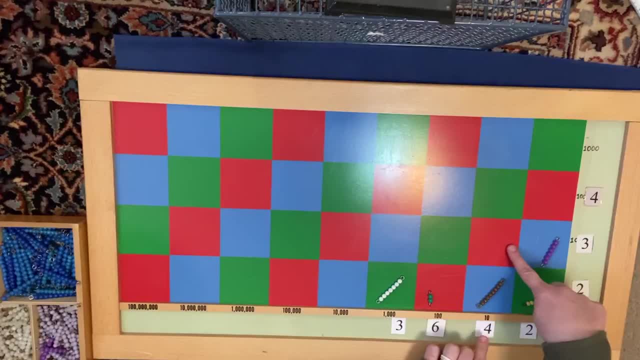 Six, This would be three times four, which is twelve. Now here, three times six is eighteen, And then three times three is nine. Don't roll on me, Okay. So we go back and make sure we have one bead bar. 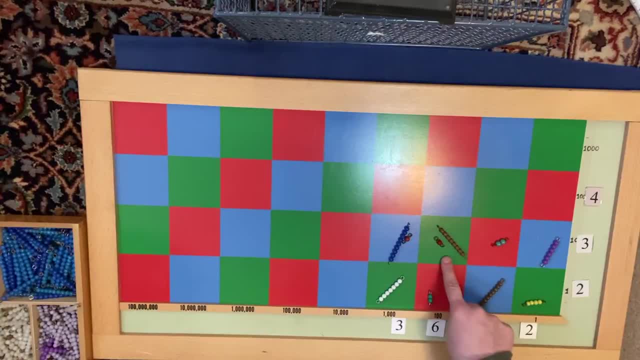 One bead bar: Yes, One bead bar, Yes. One bead bar, Yes. Eight plus one is Nine. Okay, One bead bar, Nope, We have one plus nine, which is ten Zero one. Do you remember that? 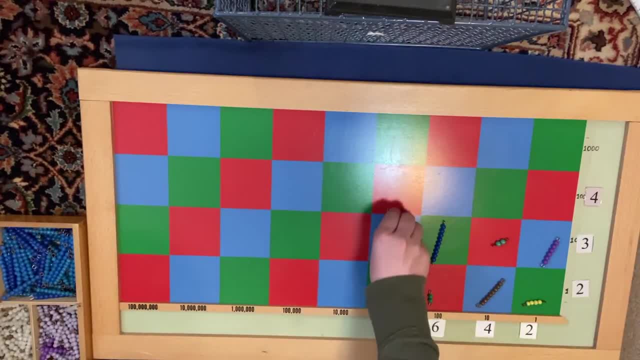 Zero with beads is just nothing, Okay. So this is exactly what we did last time. Now what we're going to do is we're going to pop from here up to here and we'll multiply all of these times four. So two times four is eight. 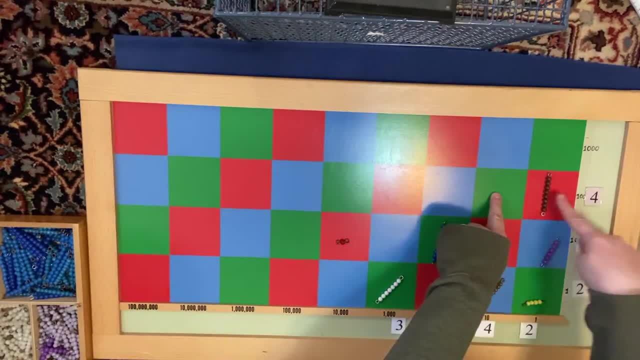 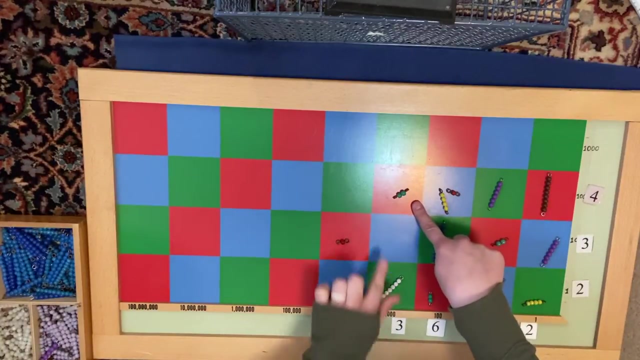 Four times four is sixteen. The six goes in the one we were multiplying. Six times four is twenty-four, And that's six One, And then 4 times 3 is 12.. Okay, so let's make sure there's one bead bar in each square. 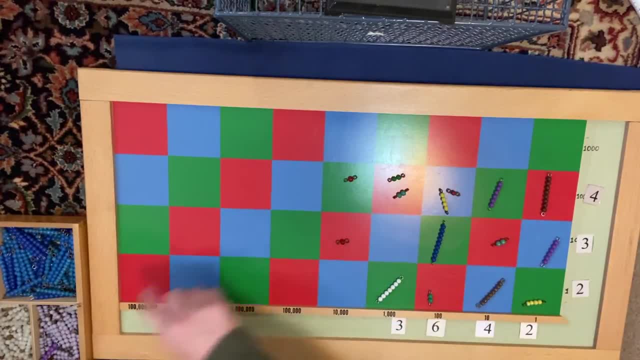 Is there one bead bar? Yes, One bead bar. Yes, One bead bar. No 4 plus 1 is 5.. One bead bar, No 2 plus 2, is 4.. Whoa, the 4 is going crazy. 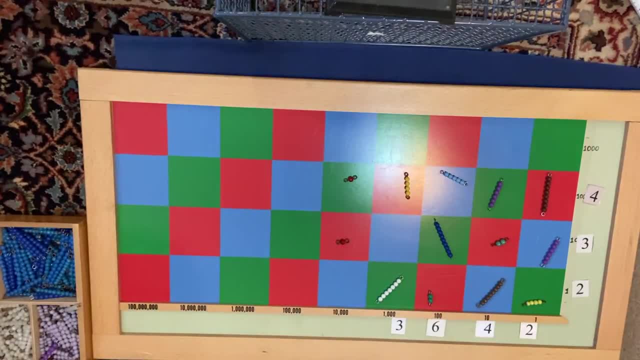 There we go. One bead bar, Okay, so we're done with our multiplication. We're done with our multiplication, but we have to get all the like categories together, So the tens with the tens, Hundreds with the hundreds, all the way down. 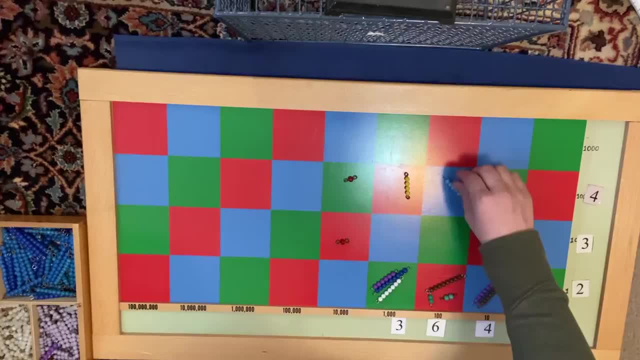 Thousands with the thousands, Ten thousands, Hundreds, thousands with the hundreds thousands- Oh my goodness, look. and a million, Whoo. So we're on the last step. This is a big number. Let's see here. One bead bar, Yeah. 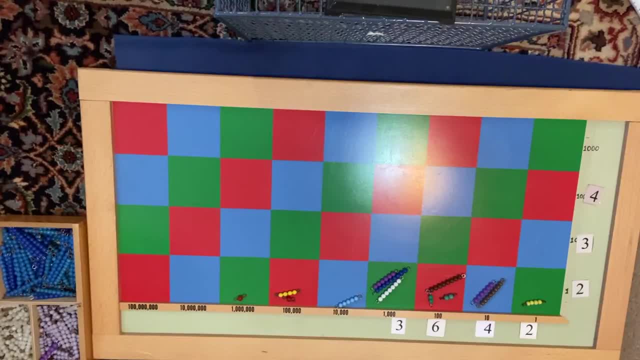 Here. No, We have to add these 8 plus 6.. What is 8 plus 6?? 8 plus 6 is 14.. Excuse me, There's 14.. Now we have to go here, Okay. 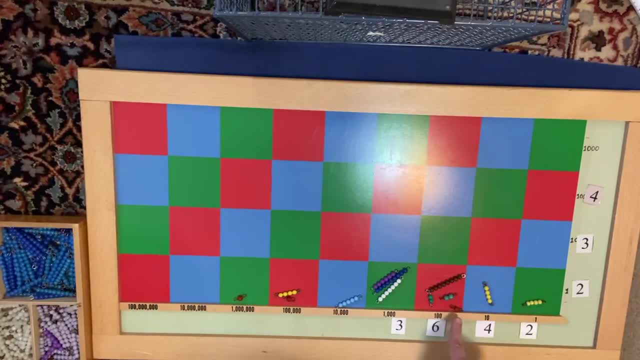 We have 8 plus 2 is 10.. 11,, 12,, 13.. So picture 13 in your head. You need a 3 and a 1.. 3 goes in the one we were counting, 1 goes next door. 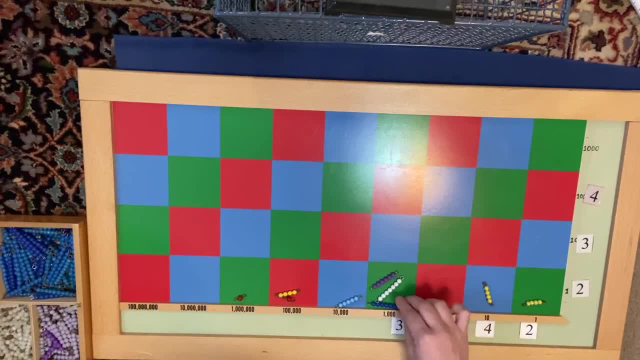 Now we need to add all this together. So 9 plus 1 is 10.. 10 plus 7 is 17.. 18,, 19,, 20,, 21,, 22,, 23.. Picture 23 in your head. 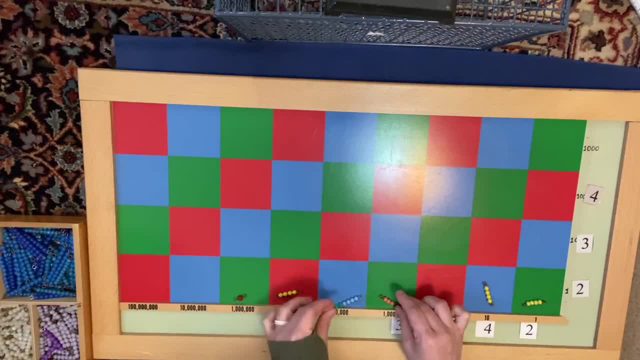 A, 2 and a 3.. 3 goes in the one we were counting, 2 goes next door. 5 plus 2 is 7.. 1 plus 4 is 5.. And then we only have one bead bar here. 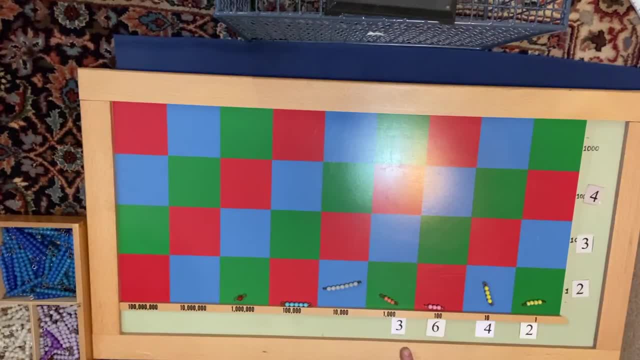 Oh my goodness. So let's count this or let's read this: 3,642.. Times 432 equals 1,573,344.. It's pretty sweet, huh? That's a big number, 1,573,344.. 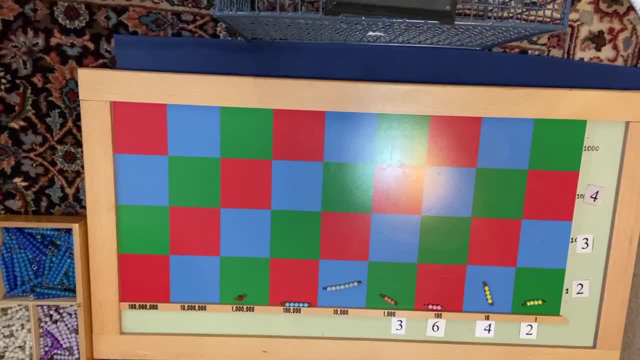 Okay, So I recommend practicing this. I think one of the most difficult things to do is to practice this. One of the most difficult parts is always putting down the final answer, making sure you do that appropriately. If you have any questions at all, please message me, email me, call me.